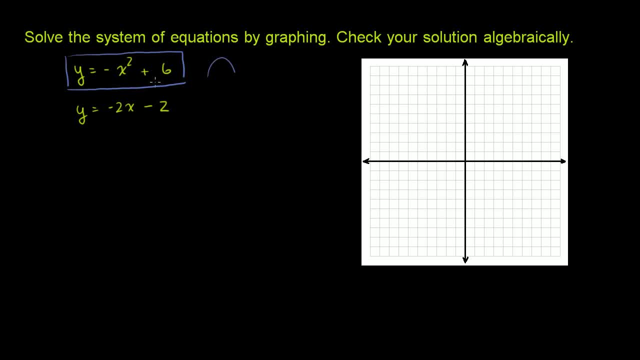 And what is going to be its maximum point? Let's think about that for a second. So this whole term right here, this whole term right here, is always going to be negative. So it's maximum, or it's always going to be non-positive. 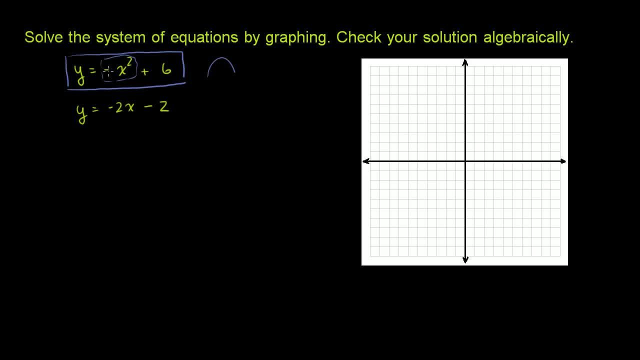 X squared will be non-negative. When you multiply it by a negative, it's going to be non-positive. So the highest value that this thing can take on is when x is going to be equal to zero. So the vertex of this parabola is when x is equal to zero. 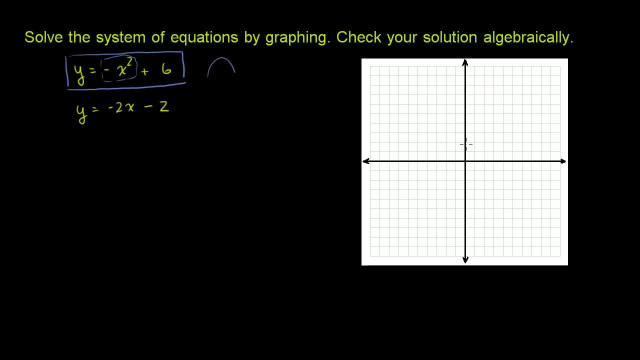 and y is equal to six. So x is equal to zero, and y is one, two, three, four, five, six. So that, right, there is the highest point of our parabola, And then, if we want, we can graph a couple of other points. 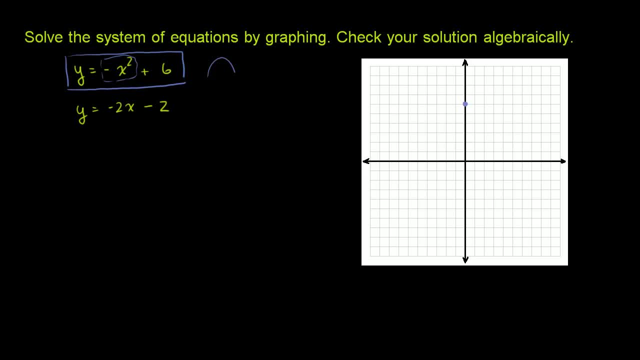 just to see what happens. So let's see what happens when. when, let's say, x is equal to. so let me just draw a little table here. So when x is equal to two, what is y? So negative x squared plus six. 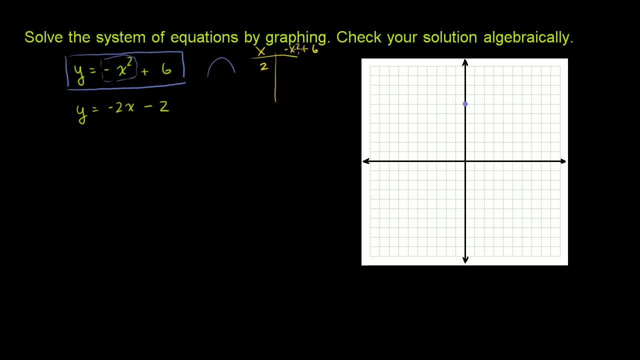 So when x is two, what is y? You have two squared, which is four, but you have negative two squared, So it's negative four plus six, It is equal to two. And the same thing when x is negative two, because you put negative two there, you square it. 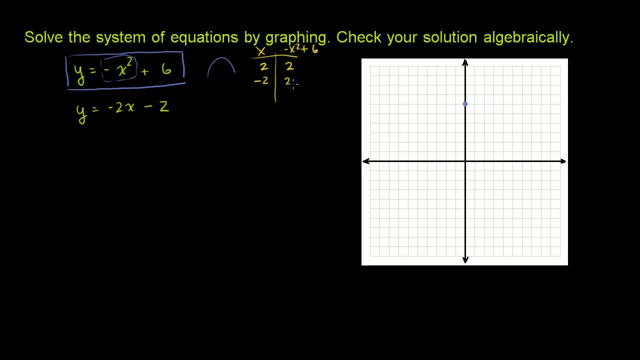 Then you have positive four, but you have a negative there, So it's negative. four plus six is two, So you have both of those points there. So two comma two. so two comma two. And then you have negative two comma two. 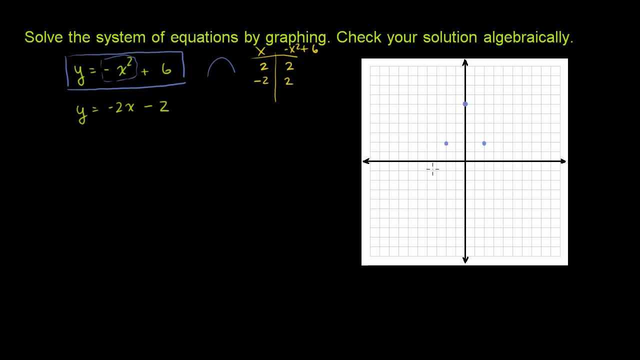 Negative two comma two, And then, if I were to graph it, I could even do a. let's try it with three as well. So if we put a three there, three squared is nine, Then it becomes a negative nine plus three. 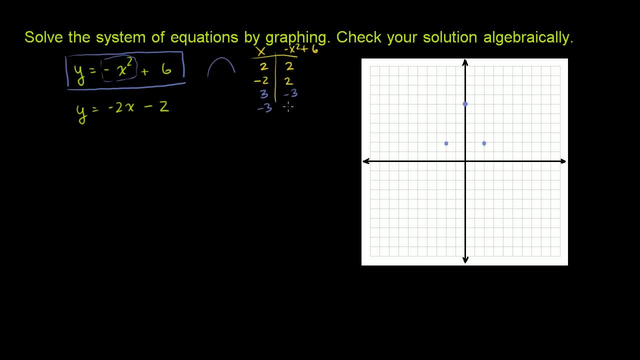 It becomes negative three And negative three will also become a negative three. Negative three squared is positive nine. You have a negative out front. It becomes negative nine plus six is negative three. So you have negative three, negative three, And then you have three negative three. 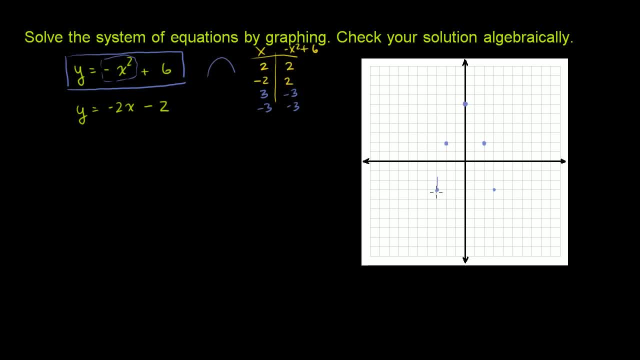 So those are all good points, And now we can graph our parabola. our parabola will look something. Oh, I was doing well, until that second part, Let's see. our parabola will look something like that. 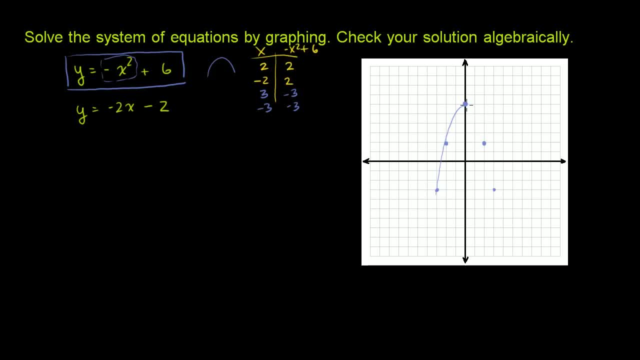 Let me just do the second part. That second part's hard to draw something, Parabola, almost. let me do it from here. Almost it looks something like that There. well, no, Let me connect this dot right here. 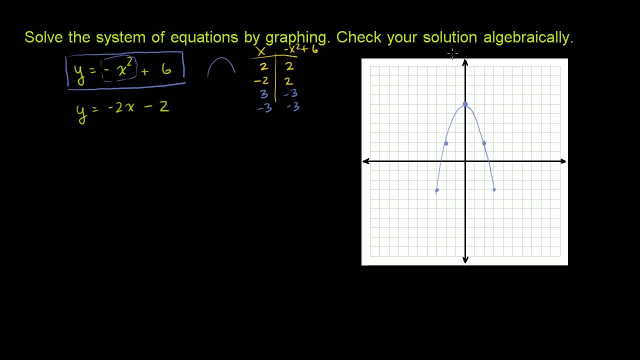 And then let me connect this. So it looks something like that. That's what our parabola looks like, And obviously it keeps going down in that direction. So that's that first graph. Now let's graph this second one over here. 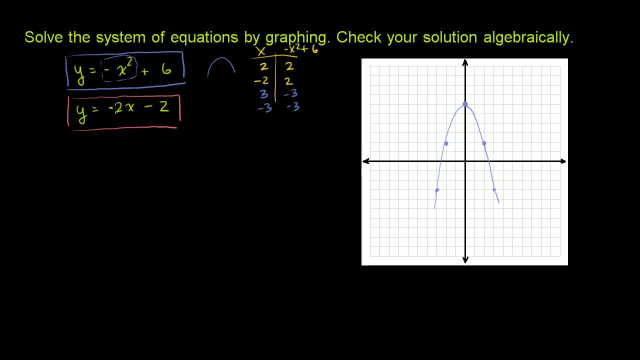 Y is equal to negative two x minus two. This is just going to be a line. It's a linear equation. The highest degree here is one. So our y-intercept is negative two. So zero one two: Our y-intercept is negative two. 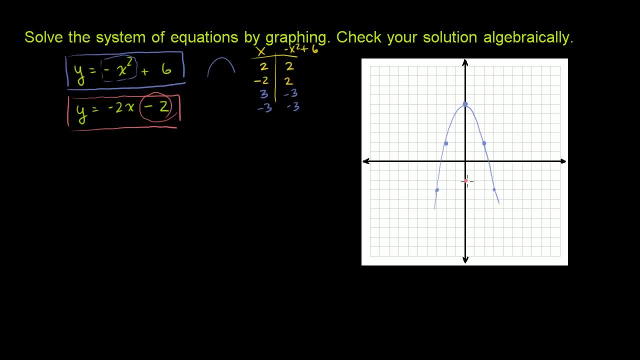 And our slope is negative two. So if we move one in the x direction, we're gonna go two in the y direction. If we move two in the x direction, we're gonna move down four in the y direction, We're gonna move down four. 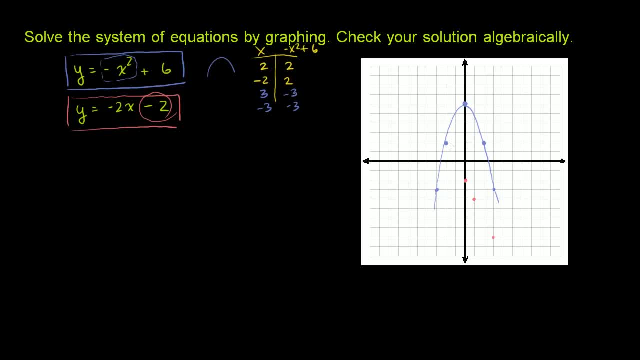 If we move back two, we're going to move up two in the y direction And it looks like we found one of our points of intersection And let's just draw that line. So that line will look something like- it's hard for my hand to draw on that. 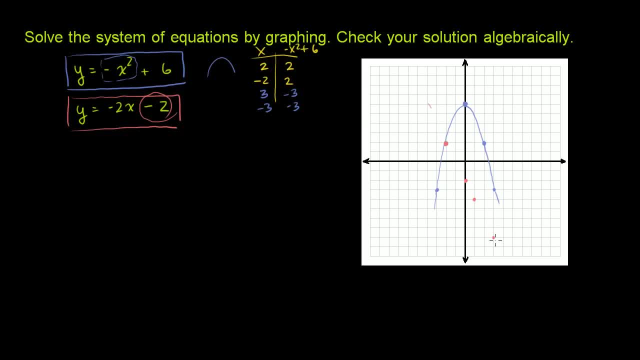 Let me try as best as I can. So it will go something. my hand is having my tablet, The hardest part. It will look something like that right there, And so the question is: where do they intersect? Well, one point of intersection does immediately pop out at us. 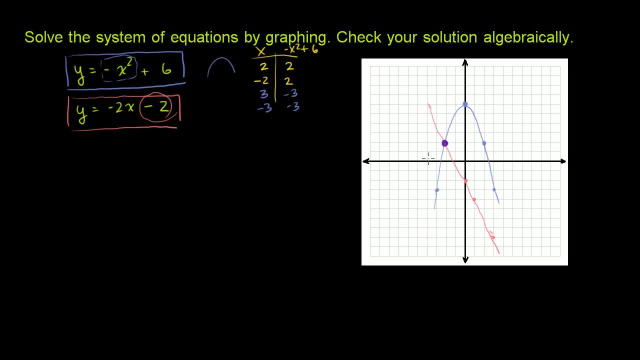 They asked us to do it graphically. That point right there, which is the point negative two, two, Which is the point negative two, two, seems to pop out. So this is the point negative two, two, And let's see if that makes sense. 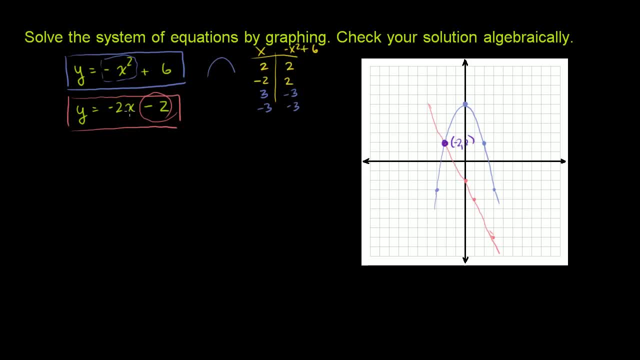 When you have the point negative two. well, when you put x is equal to negative two here, negative two times negative two is four minus two. y is equal to two. When you put negative two here, y is also equal to two. 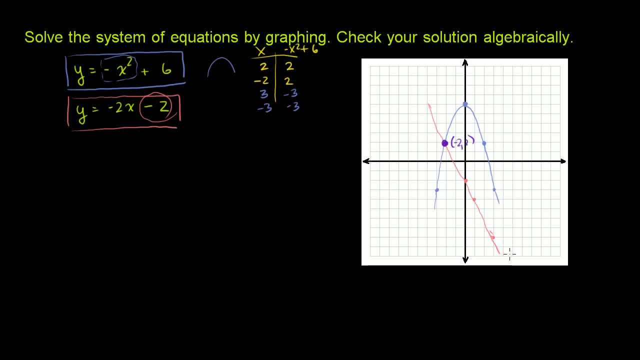 So that makes sense. And then there's going to be some other point way out here where they also intersect. There's also going to be some other point way out here if we keep making this parabola. Let's see when y is equal to positive four. 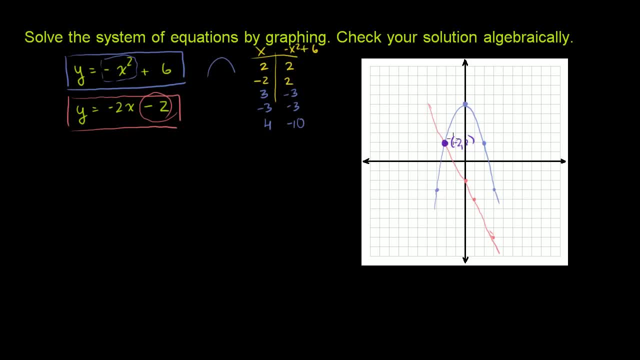 then you have negative 16 plus six, you get negative 10.. So positive: one, two, three, four, and then you go down 10.. One, two, three, four, five, six, seven, eight, nine, 10.. 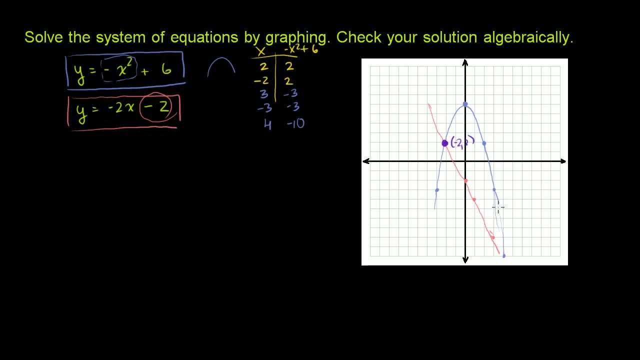 That looks like that might be our other point of intersection. So let me draw, let me connect this right there, And then our other point of intersection looks to be right there. If we just follow this red line, it looks like we intersect there. 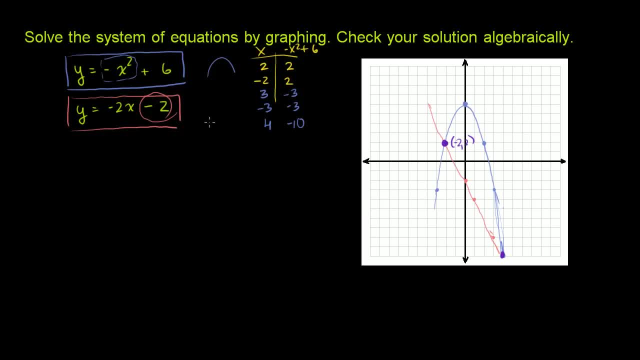 And let's verify that it works out. So four negative 10.. We know that it's on this blue line, Let's see if it's on this other line. So negative two times four minus two, That is negative eight minus two. 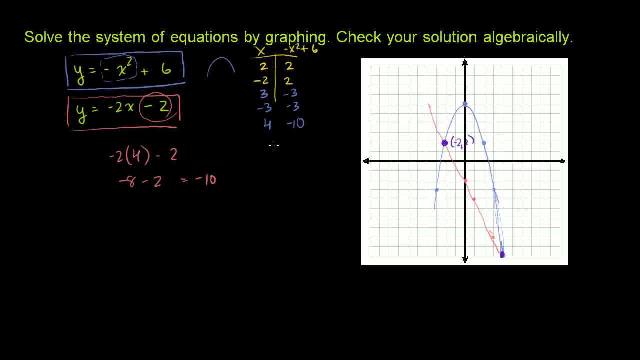 which is equal to negative 10.. So the point four: negative 10 is on both of them. When x is equal to four, y is negative 10 for both equations here. So they both definitely work out. Today we answer the second part of that one-part question that 11.3 answered, like the first half. The first. the question was: can we multiply vectors? We know we can add them, we know we can subtract them and we know kind of that we can multiply them with this thing called the. that's right. the second half of the answer: 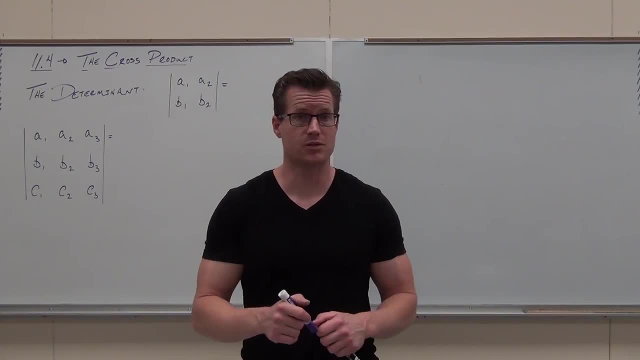 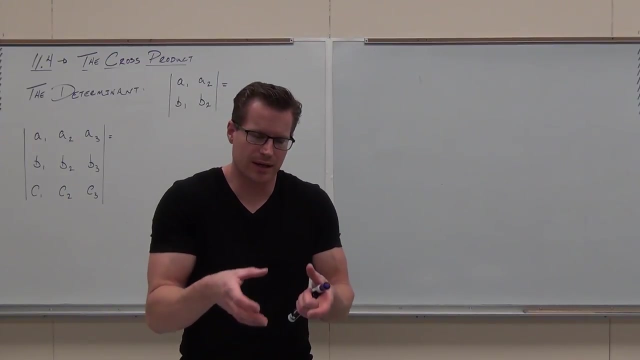 to. can we multiply them is yes, we can. One way, dot product, The other way, a different type of product is called the cross product. Now, what the cross product is, you're going to find out. And it's actually the cross product makes a lot more sense just in what it is, when we do the computation. 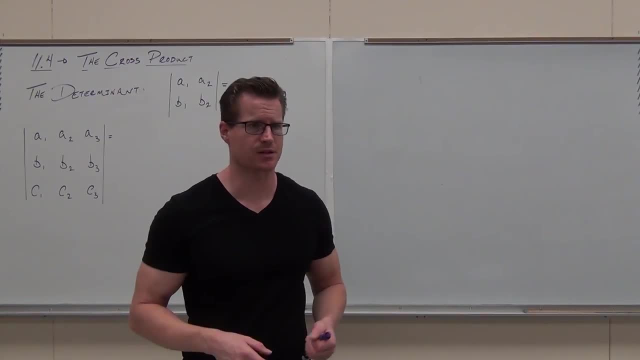 Dot product was like: okay, we get this number, what's the number? And we spent an entire class discussing what that number was and how we use that number. Cross product: when you see what it does, it's going to be like: 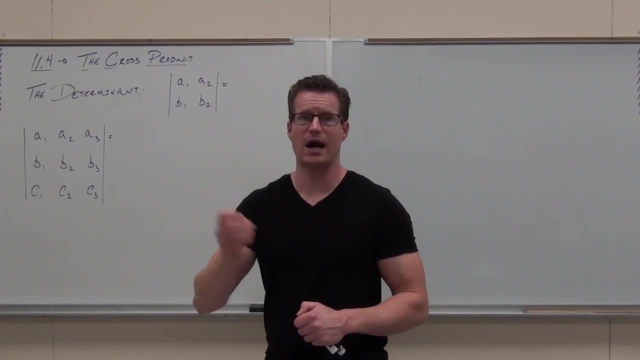 okay, I get it. I understand what this is. It makes something actually graphable relevant that you're going to get. Before we get on into how to actually compute the cross product of two vectors, I've got to talk about determinants.